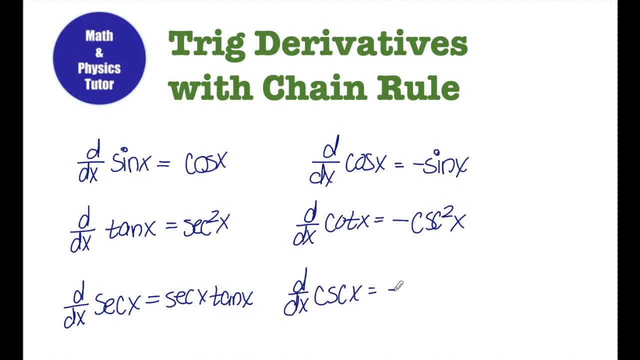 of cosecant x. this is also negative. the derivative of secant was secant x, tan x. so the derivative of cosecant x is cosecant x, cotan x. So the derivatives of all the co-functions are negative and they come kind of from the derivatives of these other ones. You can derive: 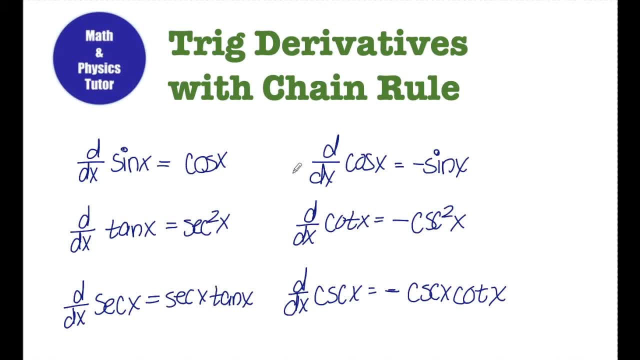 all of these four trig derivatives based on just sine and cosine. but it's a little lengthy and you don't want to have to do that for each example, so you're definitely better off just memorizing these six trig derivatives. Let's look at a couple of examples of finding derivatives. 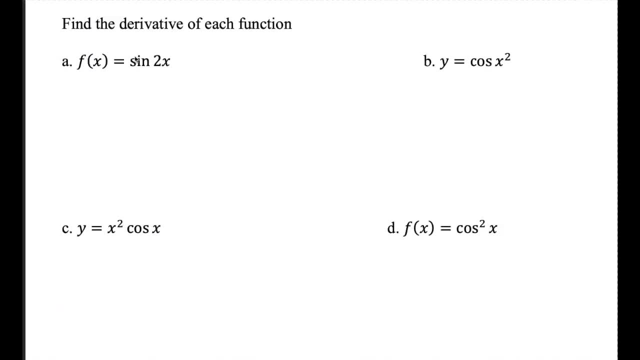 of trig functions with and without the chain rule. Part a f of x is equal to sine of two x, So I can see here that I'm taking the sine of two x. We learned on the previous page that the derivative of sine x is cosine x. but since I'm not taking sine of plain old x, I need a chain. 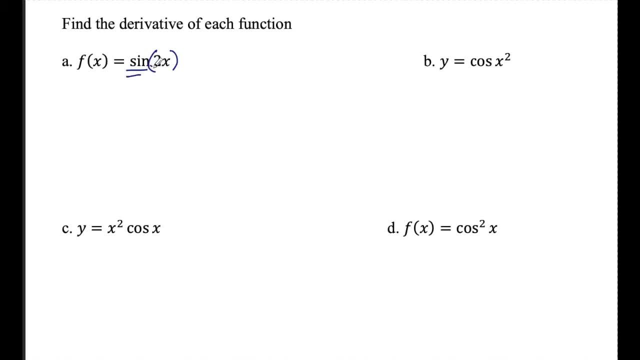 rule. here I'm going to look at sine as the outside and the two x as the inside. So when I find f prime- remember the chain rule says: derivative of the outside, leave the inside alone times the derivative of the inside. If that doesn't work, I'm going to look at the 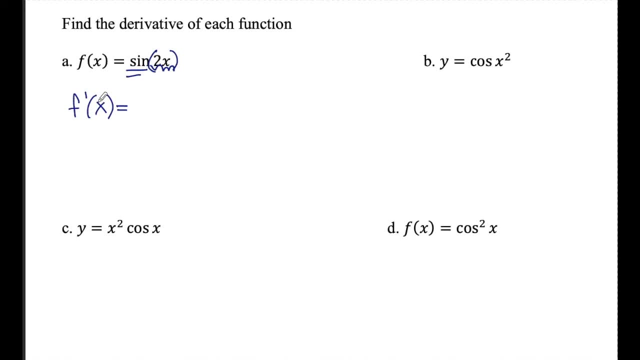 chain rule video which explains how those words apply to the chain rule. So the derivative of sine is cosine. I leave the two x alone and then I multiply by the derivative of the inside, which is two. I can either leave it like this or move it to the front, where you usually see it. 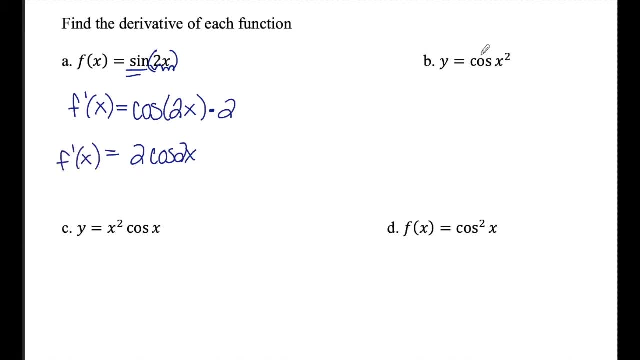 So there is f, prime Part b. y is equal to cosine x squared This square, here, this exponent, is attached just to the x, not to the whole cosine of x. So I'm going to leave the two x alone and in this case the outside is going to be the cosine, The inside is your x squared, The derivative. 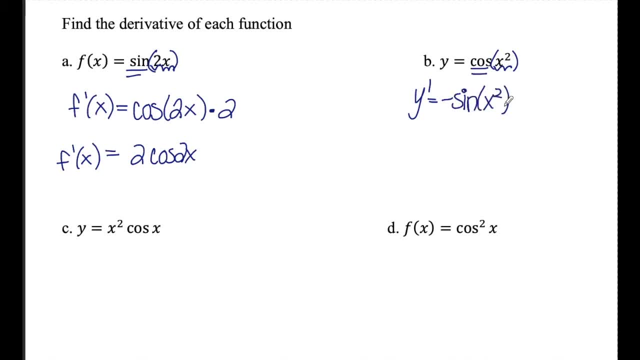 of cosine is negative sine. I leave the x squared alone multiply by the derivative of the inside. The derivative of x squared is two x. If I just rewrite that, I have negative two x sine. x squared Part c. y equals x squared cosine x. Since there's no operation here between the x. 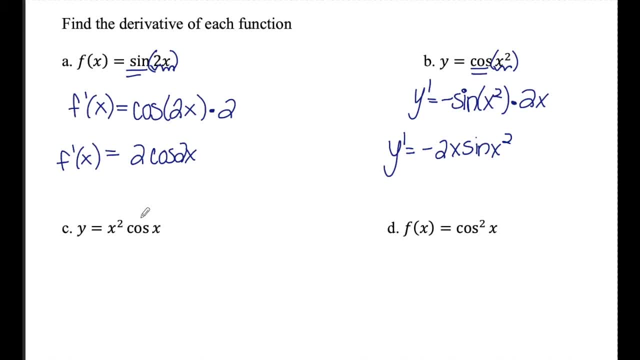 squared and the cosine x. that's implied multiplication. So since I'm multiplying x squared and cosine x, I'm going to have to use a product rule where x squared is the first and cosine x is the second. So the product rule says: first, derivative of the second: The derivative. 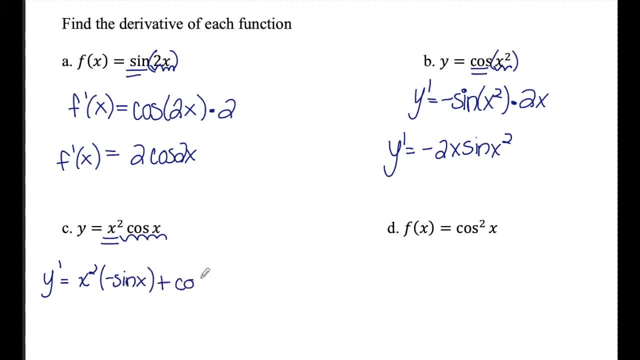 of cosine x is negative sine x plus the second, cosine x times the derivative of the first. The derivative of x squared is two x. You can leave it like this, or at least bring that negative to the front. So it says negative x squared sine x plus two x. cose x. Part d. 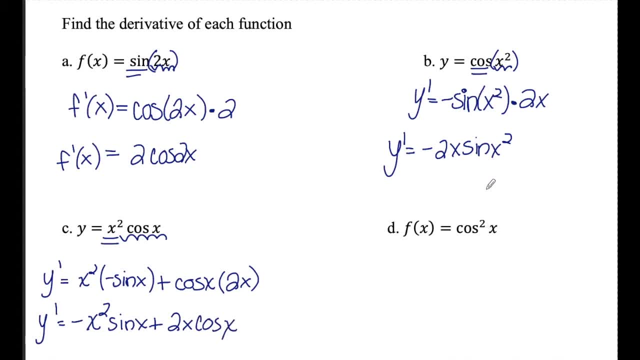 f of x is equal to cos squared x. So this is different from b. right In b just the x was being squared. This notation here is the same thing as cosine of x, that entire thing squared. So it's not just the x, it's the whole cosine x function that's being squared. So when I use the 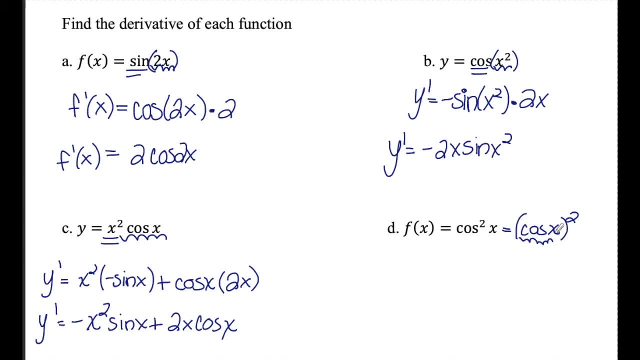 chain rule. here I'm actually going to look at the cosine x as the inside and then something squared as the outside. So when I find f prime here, I'm going to bring this exponent to the two. leave the inside alone, drop the exponent by one. So that's power rule derivative of the. 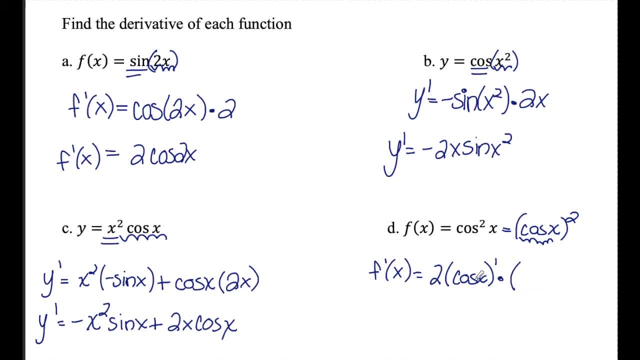 outside, leaving the inside alone, times the derivative of the inside. The derivative of cosine x is negative sine x. So f prime here is going to be equal to negative two cosine x sine x. Let's look at two more kind of easier examples like these, and then we'll go into some trickier. 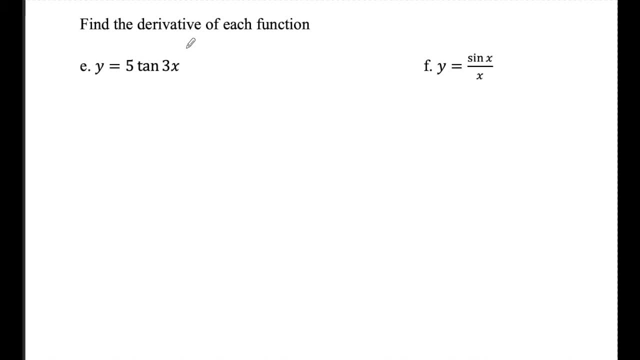 trig functions. Part e says y equals five tan of three x. In this case I have a constant times a function. So I know that when I take the derivative of something like that y prime, I can just bring down the constant and then I'm going to take. 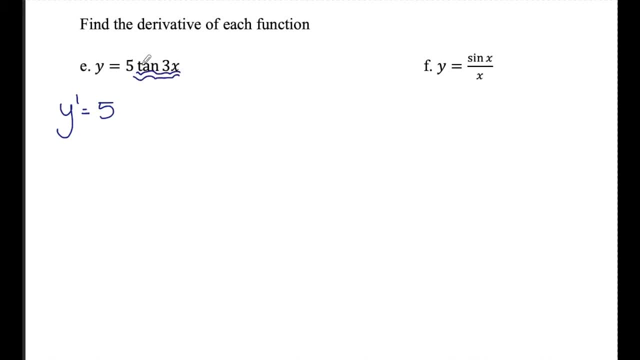 the derivative of tan of three x. For the derivative tan of three x, three x is going to be my inside and tan x is on my outside function. So the derivative of tan I know is secant squared x, but I'm not taking tan of just x, I'm taking tan of three x. So I have secant squared three x. 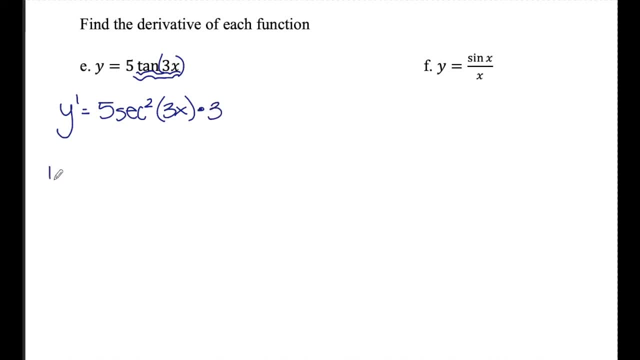 The derivative of the inside, the derivative of the three x is three, And I definitely want to simplify this and make it 15 secant squared. three x, Part f, y is equal to sine x over x. Since I have division here, I'm going to need to use the quotient rule. The quotient rule says low. 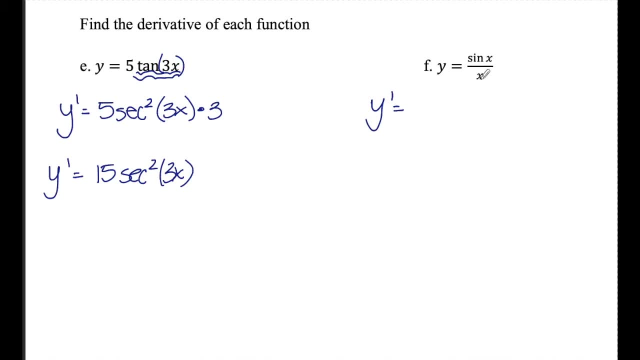 d high, low times. the derivative of the high minus high d low. derivative of the low all over low squared. So my derivative here is going to be low x d high. the derivative of sine x, cosine x minus high. sine x d low. the derivative of x is one all over low squared. 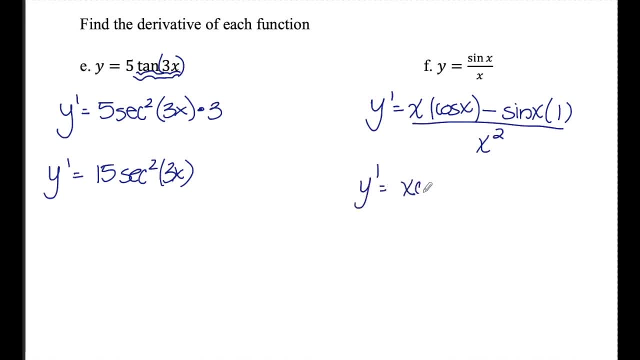 so x squared. I can clean this up just a tiny bit really, just by dropping those parentheses, So I get x cosine x minus sine x over x squared. Let's look at a trickier example where I have multiple derivative rules within one problem: Find, the derivative of the function y is equal to. 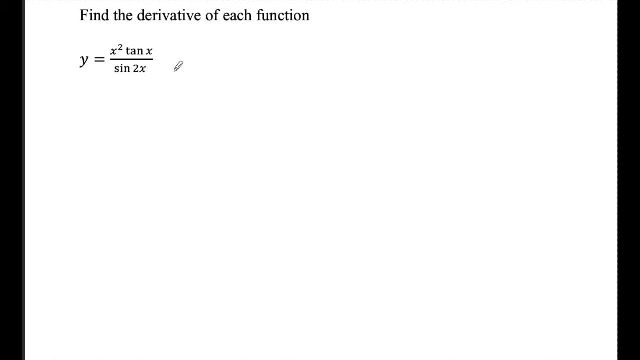 x squared tan x over sine of two x. So, first and foremost, I see that this is a quotient of functions, So I know I'm going to have to apply the quotient rule where this is the high and this is the low. So when I start to find 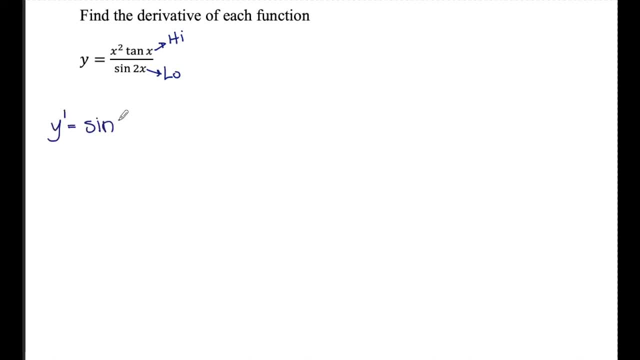 y prime. I do low, d, high, So sine two x times the derivative of the high. When I do the derivative of x squared, tan x, I'm going to need a product rule where x squared is my first and tan x is my second. So I'm going to have first x squared, derivative of the second. 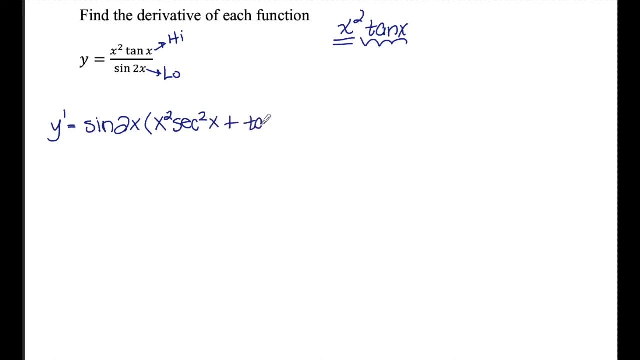 The derivative of tan x is secant, squared plus the second tan x times the derivative of the first two x. So now this is within my quotient rule: Low, d high minus the high is x squared tan x and now d low. So when I take the derivative of sine of two x, I need a chain rule where sine 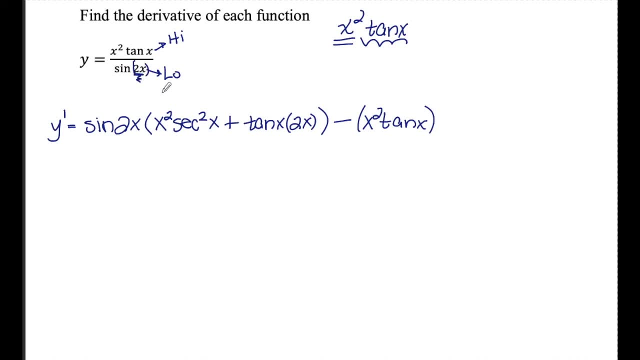 something is my outside function and then the two x is the inside. The derivative of sine is cosine. I leave that two x alone Times the derivative of the inside. The derivative of two x is two. So this takes care of the numerator in my quotient rule. This whole thing is going to be over low squared, So 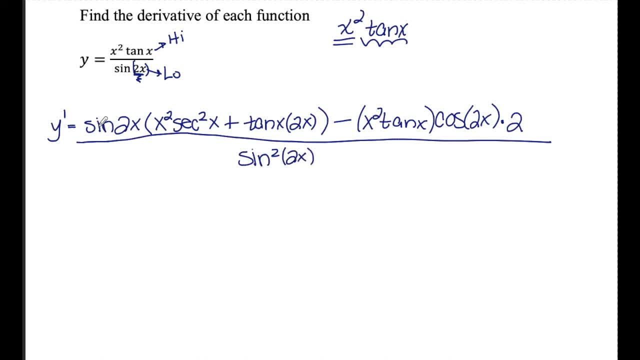 sine squared two x From here I'm going to simplify the numerator a little bit. I'm not going to do anything so crazy. I am going to distribute the sine of two x in here so that I have x squared sine two x secant squared. 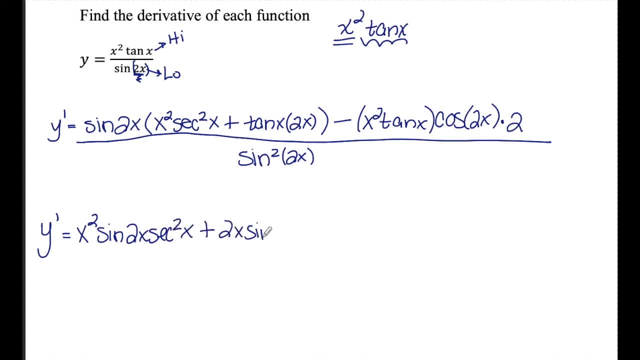 x plus two x, sine, two x, tan x. That takes care of this first piece. And then here this is just all multiplication. So I'm just going to write this as one giant term: minus two x squared tan x, cos of two x, That whole thing over sine squared two x. This is super messy, Don't worry so much. 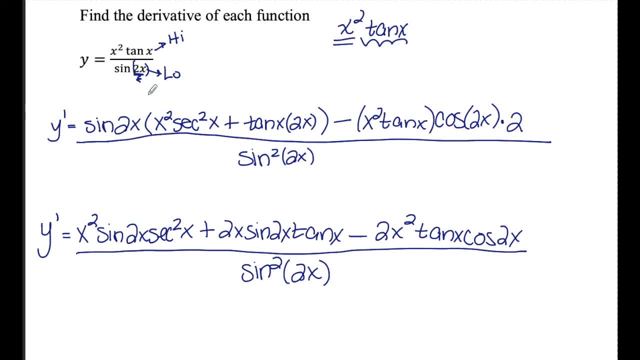 about simplifying these or trying to make them look any nicer. As long as you're able to do it, as you can apply the rule and get to here, you're good to go. Once we start looking at applications with trig derivatives, they're not going to be something so messy like this. 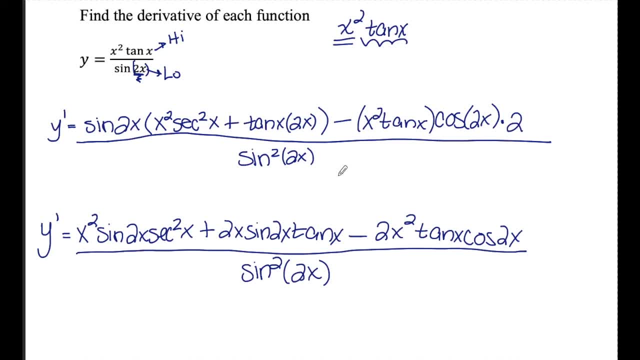 It'll be something a little bit nicer, But just to get a hang of all the different differentiation techniques, we want to be able to at least get to this step. Let's look at one more example of a trig derivative with a chain rule. 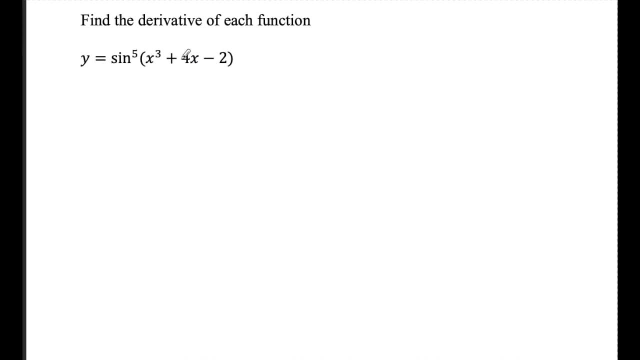 Find the derivative of the function. y equals sine to the fifth of x cubed plus four x minus two. This is the same thing as sine of x cubed plus four x minus two. This whole thing raised to the fifth power. So this is actually going to be a chain rule within a chain rule. So first I'm going to look. 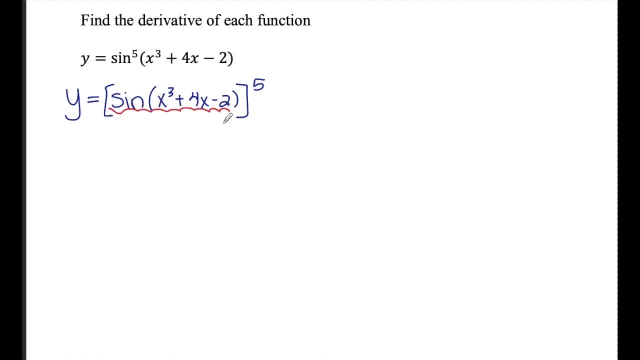 at the sine of x cubed plus four, x minus two. This is going to be my inside and something to the fifth is going to be the outside. So I'm going to start by bringing the five to the front using the power rule. So five to the inside, And then I'm going to start by bringing the five to. 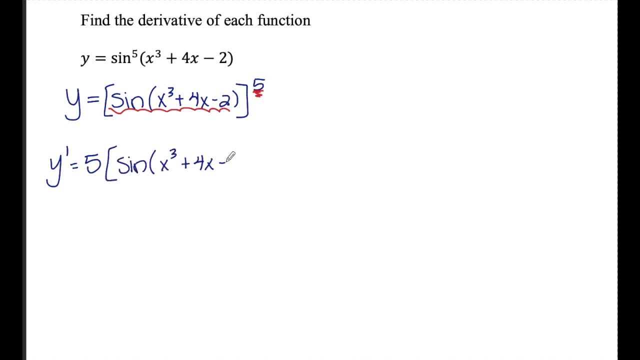 the front. Leave that inside alone. Drop the exponent by one. So that's derivative of the outside. Leave the inside alone. But since this thing was my inside, now when I take the derivative of sine of x cubed plus four, x minus two, I need to use a chain rule again This time where sine: